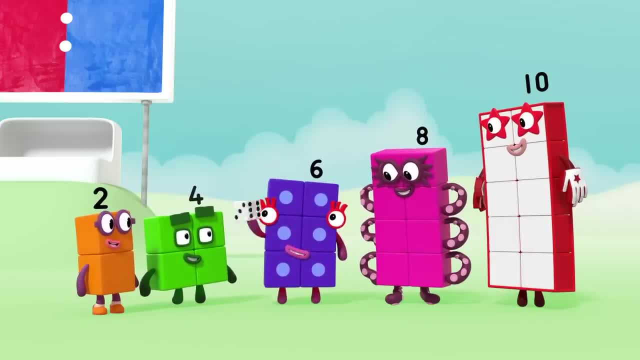 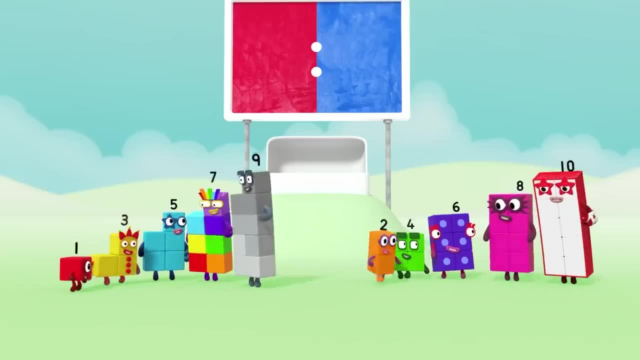 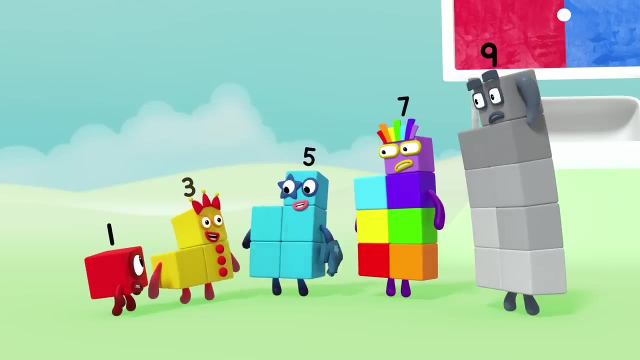 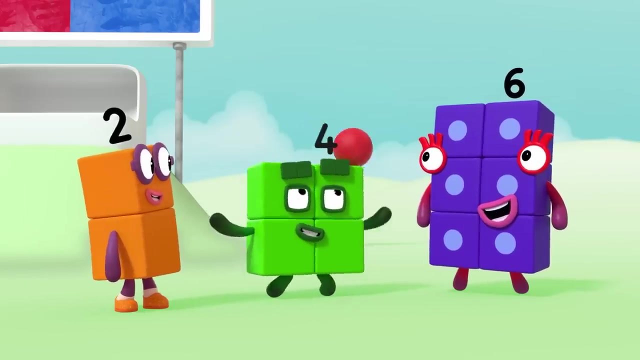 Picking sides and playing games. Both our teams need funky names. That's a great idea. Six: Each team think up a name. We can be the Yellows, But we're not all yellow. Oh right, Hey, look, Roll, roll, Easy. Watch me See. 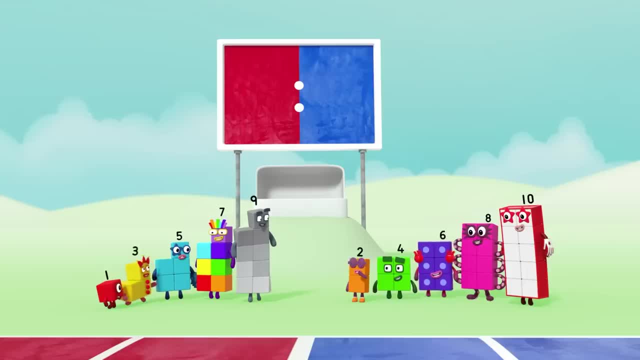 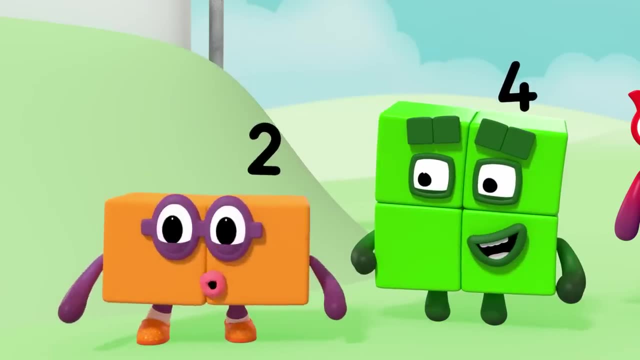 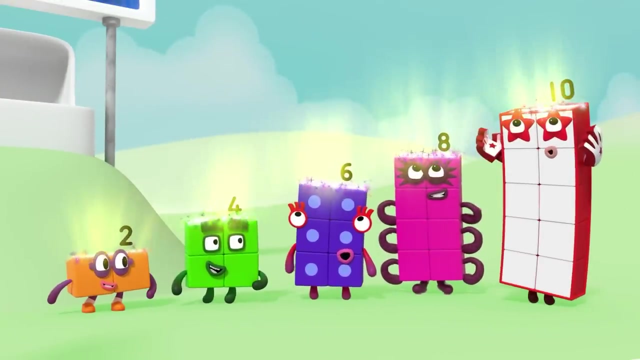 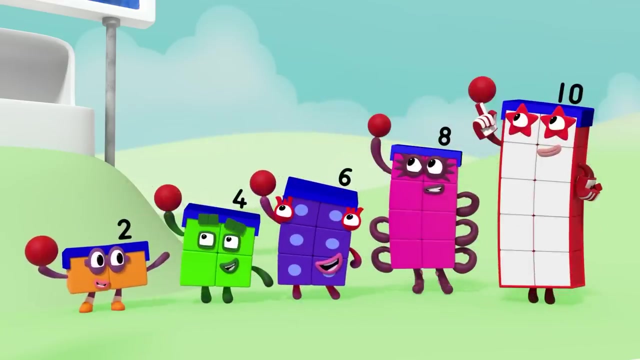 Not fair. We don't all have big, flat, even tops like you. That's it. When we stand two blocks wide, everyone on my team does have an even top, See, So let's call ourselves the Even Tops, Go Evens. 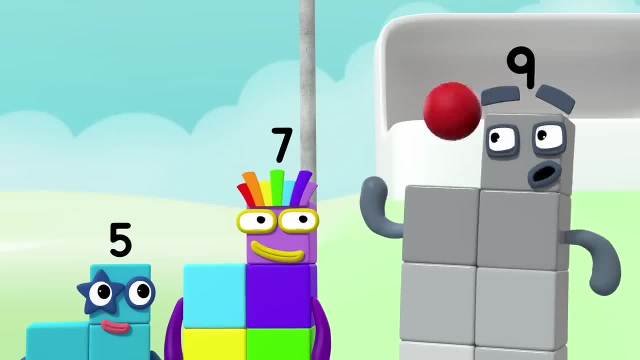 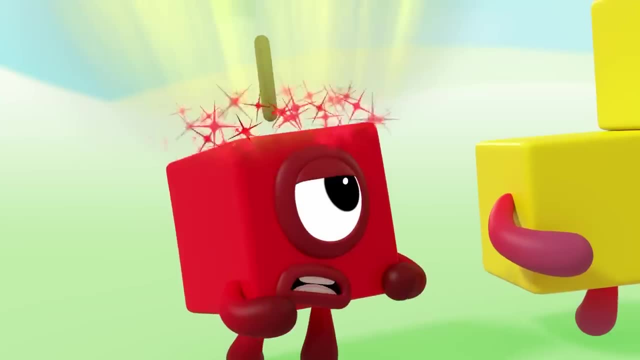 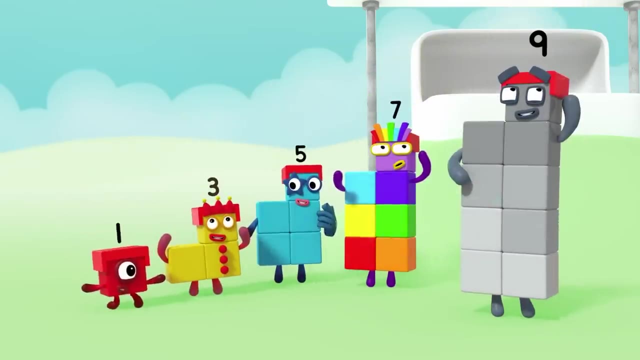 What, What, What, What, What, What, What. None of us have flat tops. We've all got one odd block sticking up. Hey, You know what I mean. All right, then Let's call ourselves the Odd Blocks. 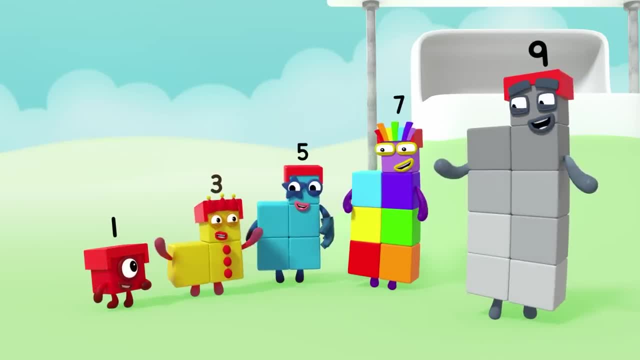 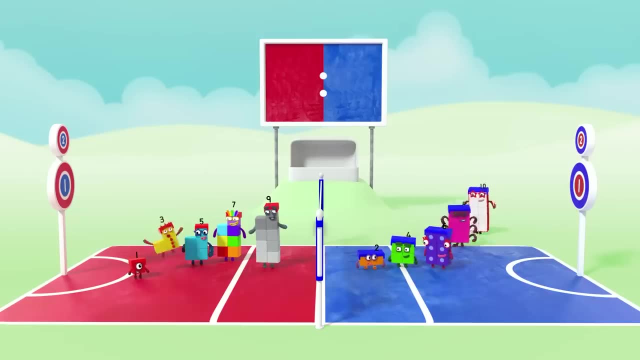 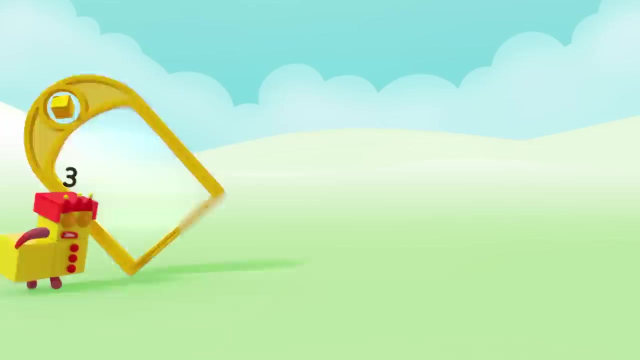 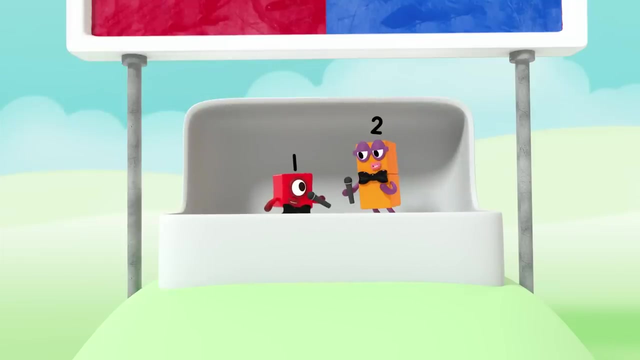 Go Odds. Let's play bounce ball Odds with me. Evens over here. Wait, wait, wait. Huh, Who's going to keep score? I know What's this: One for the Odds, Two for the Evens. 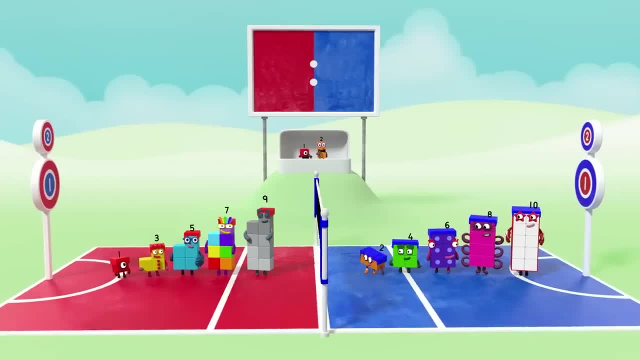 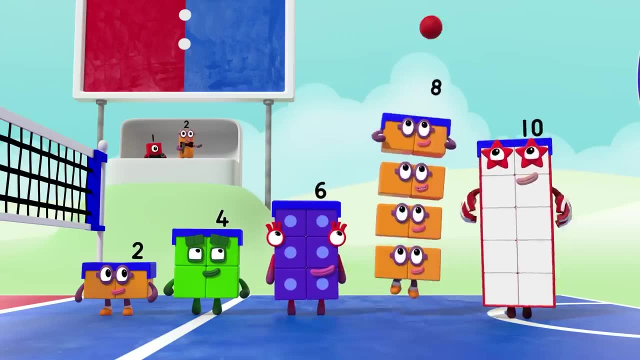 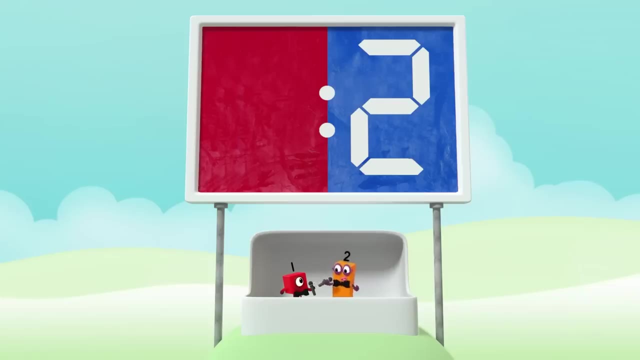 Let's play bounce ball. We're off to a great start. The ball is with the Even Tops And it's two, four, six, eight, ten. A great shot. my turn. Two points to the Evens. Now let's see that again in slow motion. 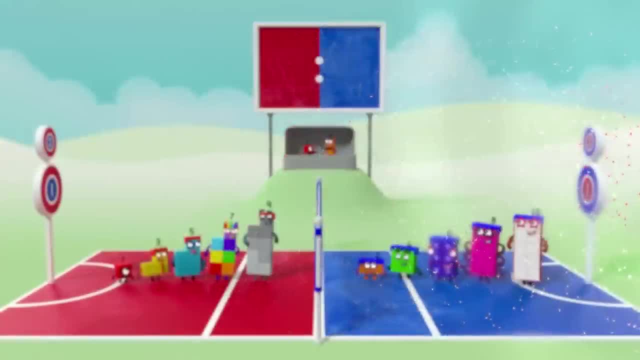 Look at that: Two, Two, lots of two. Two, lots of two. Three, lots of two. In fact, each of the Evens is two more than the one before. Let's see what the Odd Blocks can do: One, Three. 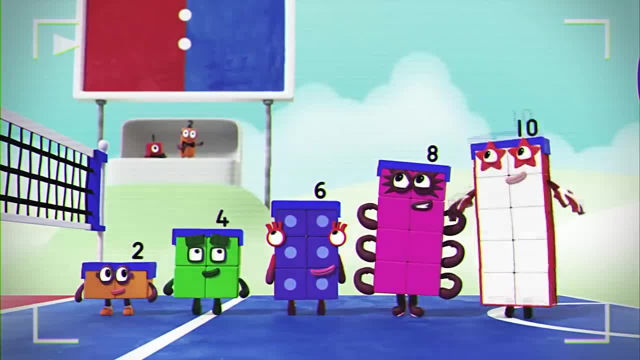 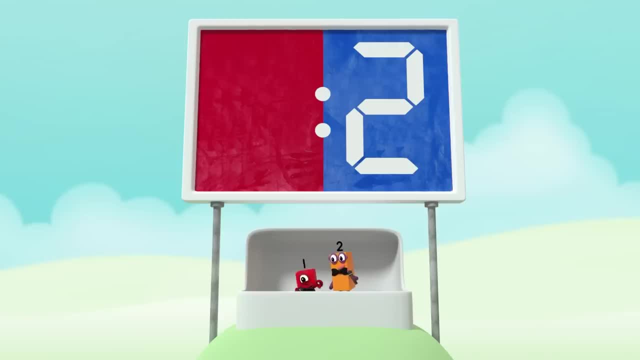 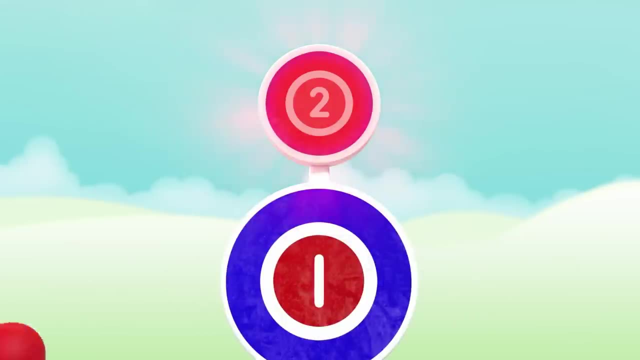 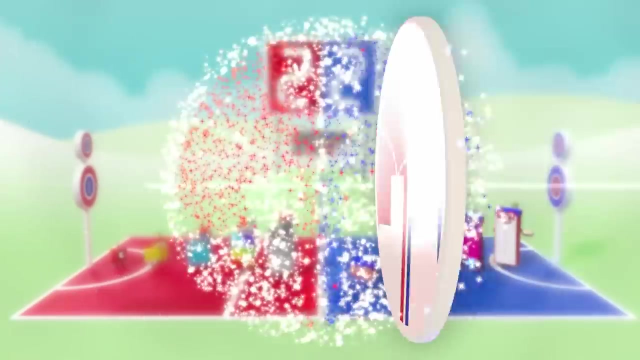 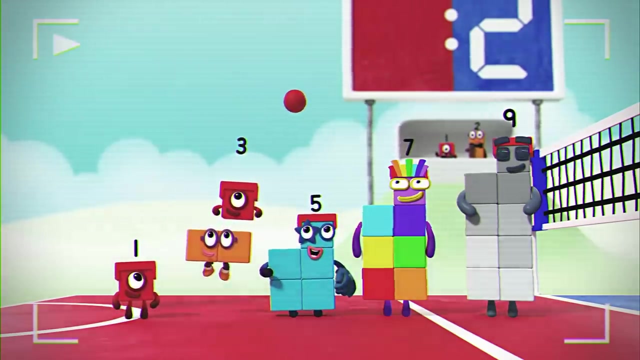 Five, Seven, Nine. Amazing Two points to the Odds. That makes the score seven-none. One, One, Two, Three. It started with one and there she is again on top of two, making three, and again on two, twos. 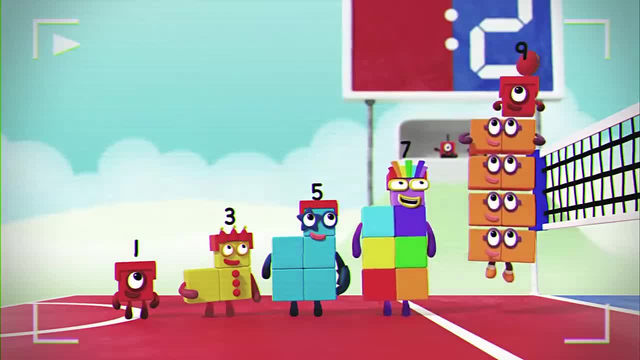 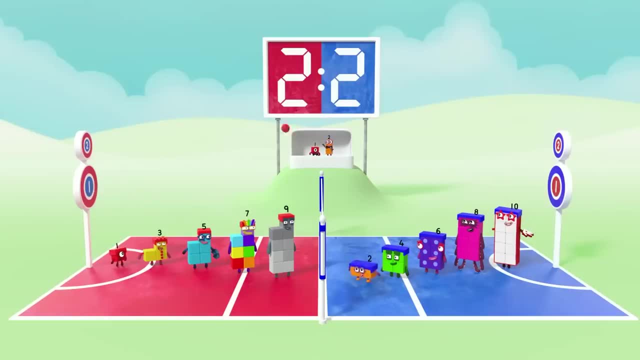 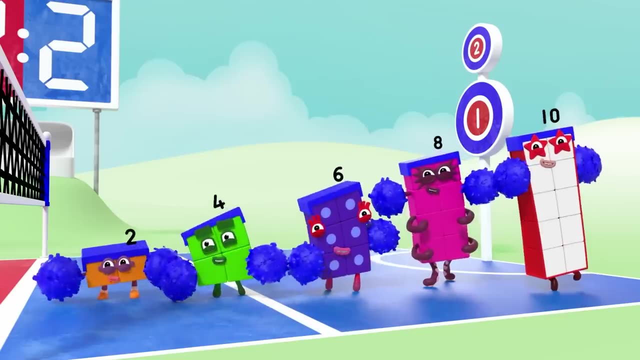 Look, each of the odds is two more than the one before, with an odd one sticking out on top With the score level. it's all to play for. What can they do now? Three, two, three, two, four, six, eight, ten. 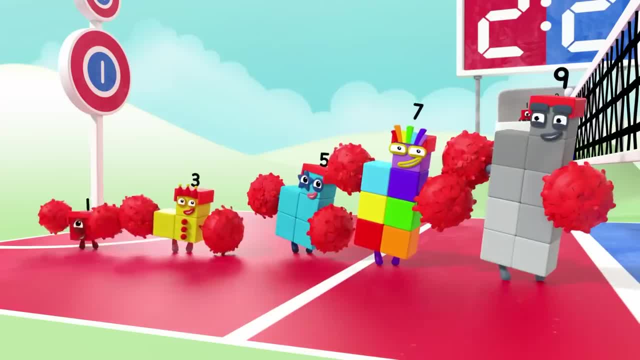 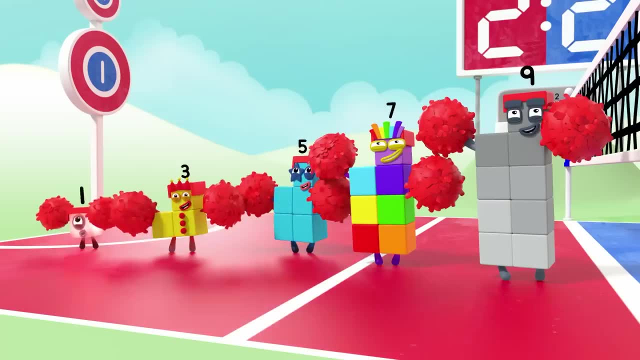 Come on, even score again. Ten, eight, six, four, two. That's what even numbers do. One, three, five, seven, nine. We are odd and we feel fine: Nine, seven, five, three, one Odds are having so much fun. 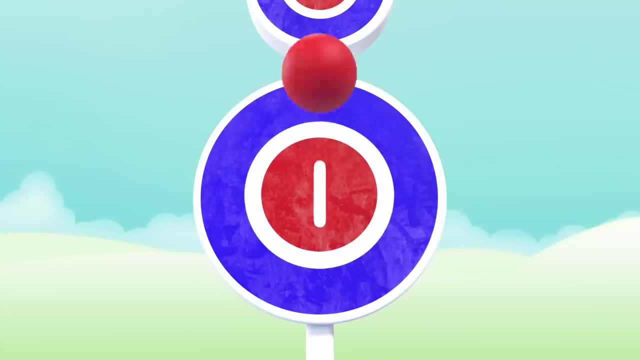 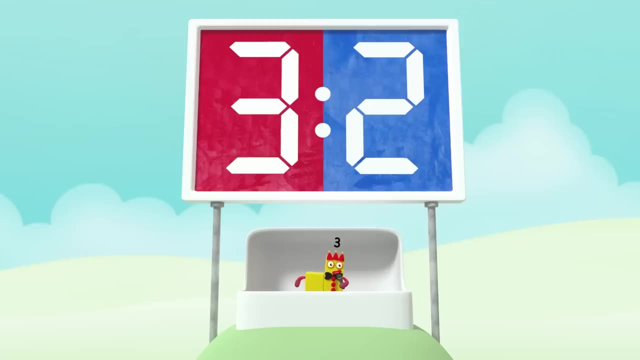 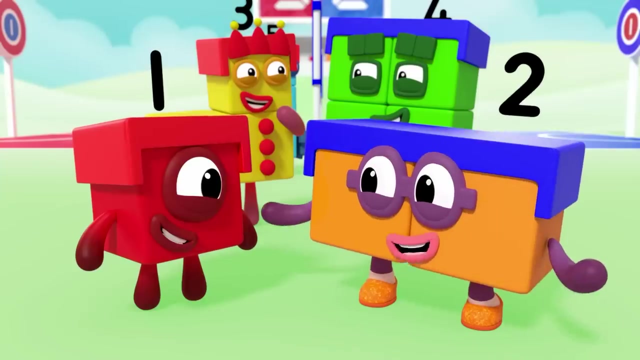 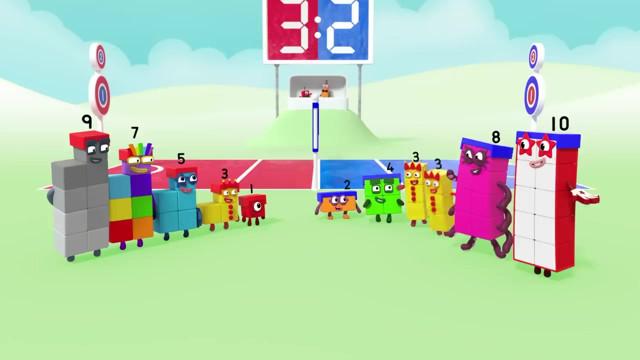 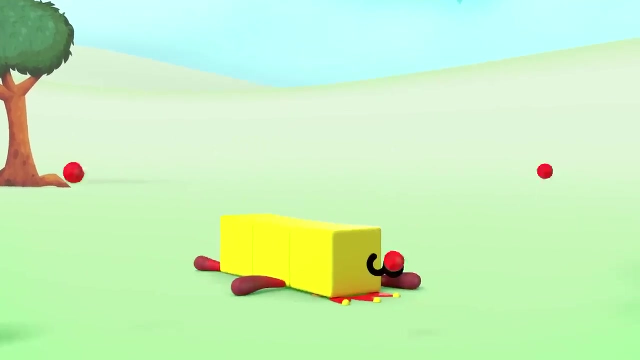 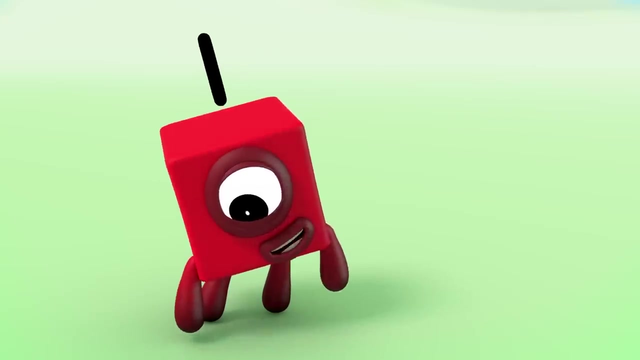 The odd bloc's beat them. That's all they need now. Aw, beat the even tops by a magnificent three points to two. what can I say? even we couldn't beat the odds. well, if you can't beat them, I wish I could be you. seven. you're so lucky you can be me. just ask a friend to jump on. 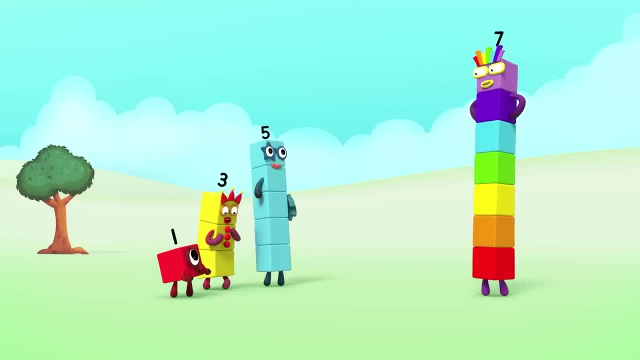 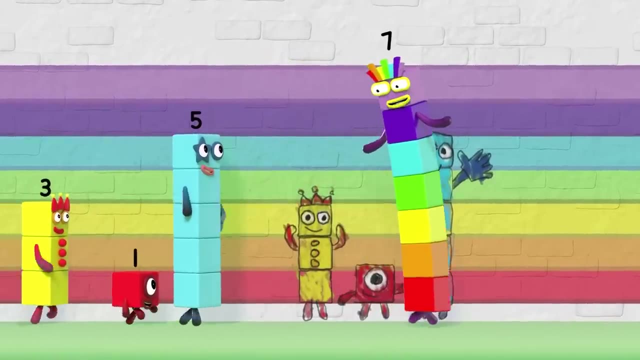 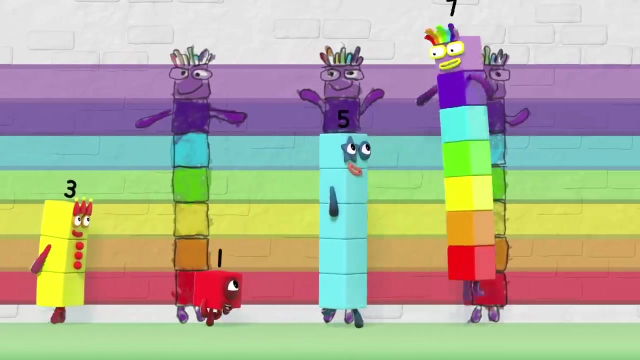 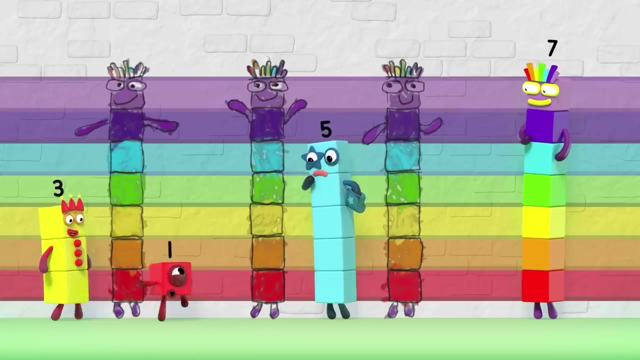 your head. but first you have to know the difference between you and me. we all have a place, but we're different. that's very easy to see. we're all friends here, but we're different. but what makes you you and not me? I'd love to be you, but I come up short. I need to add something, but what? 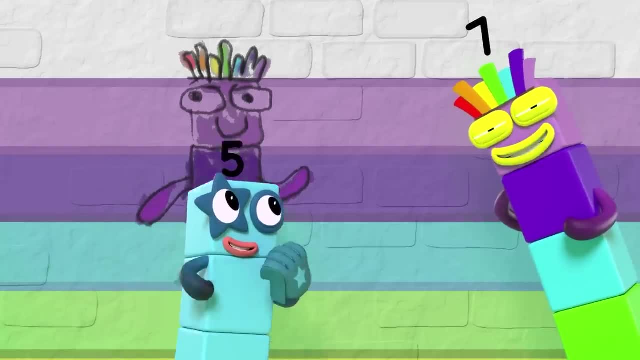 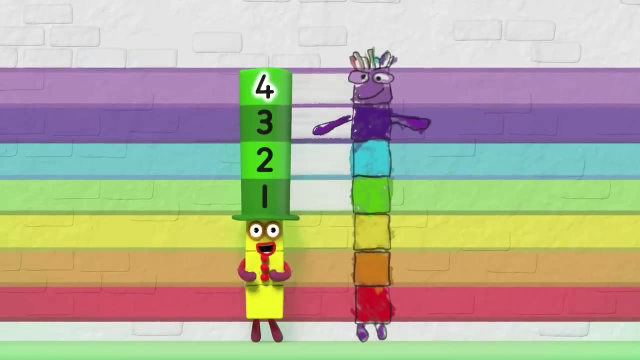 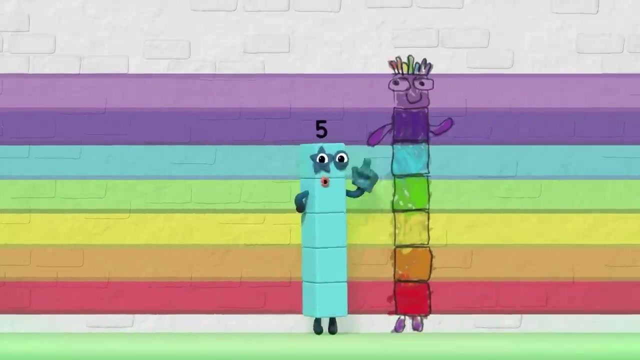 I'd love to be lucky like seven. what have you got that we haven't got? I could try on a hat, that's the difference. or I could stand on a box. that's the difference. that's the difference. that's the difference. and if the difference won't pop into your head, you can count the missing blocks: one, two, two, the. 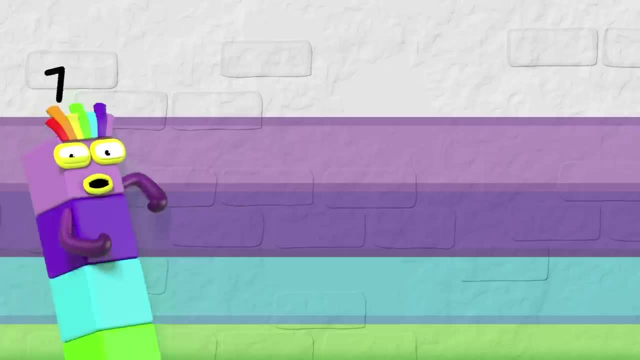 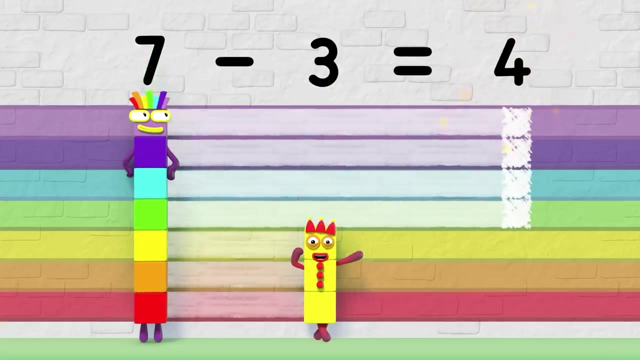 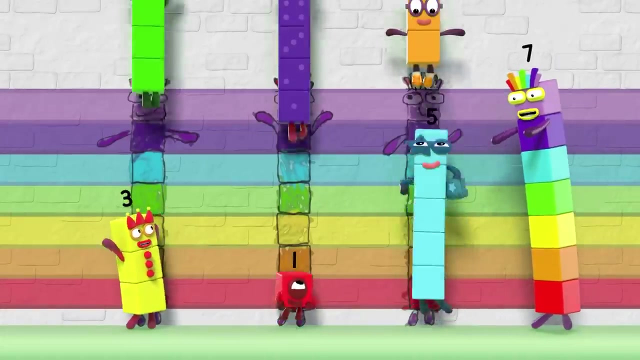 difference is two. so what's the difference? seven minus three equals four. that's the difference. four. seven minus me equals six. that's the difference. six. seven minus five equals two. that's the difference. so make up the difference and everyone will see what the difference is between you and me. 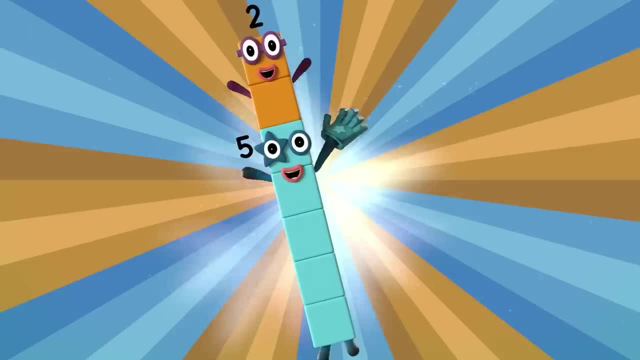 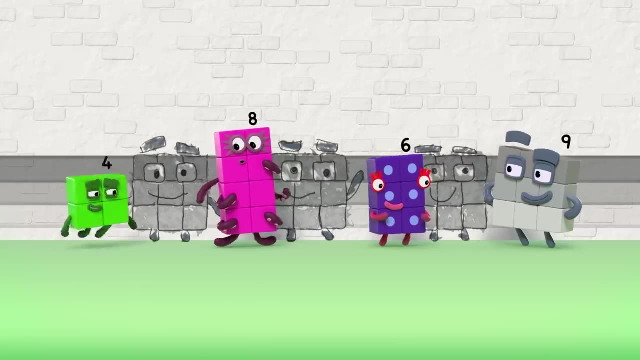 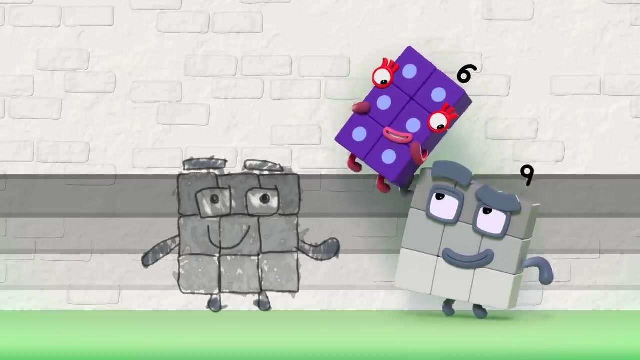 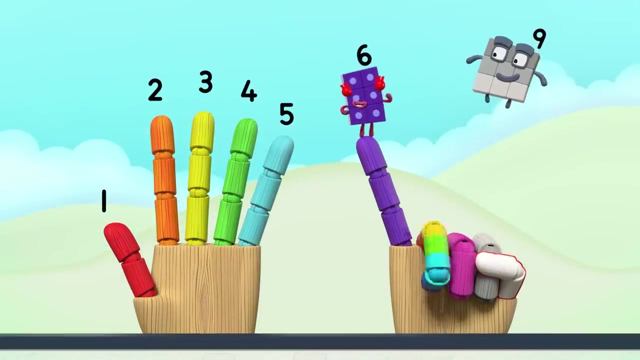 I'd love to be you, but I come up short. I need to add something. but what I'd love- to be stronger like nine- is: what have you got? if we haven't got, you can count on your hands. seven, eight, nine, that's the difference. three, one, two, three. 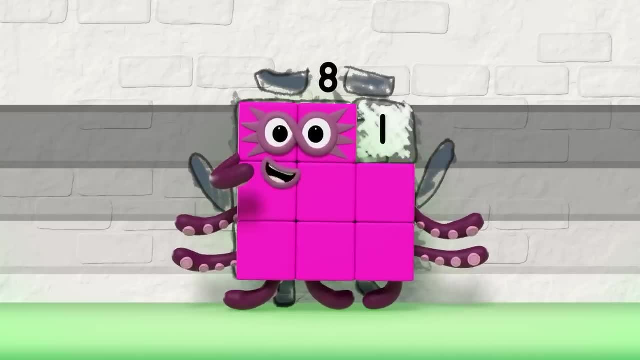 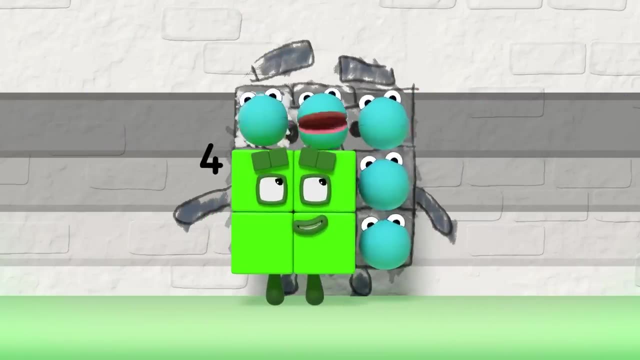 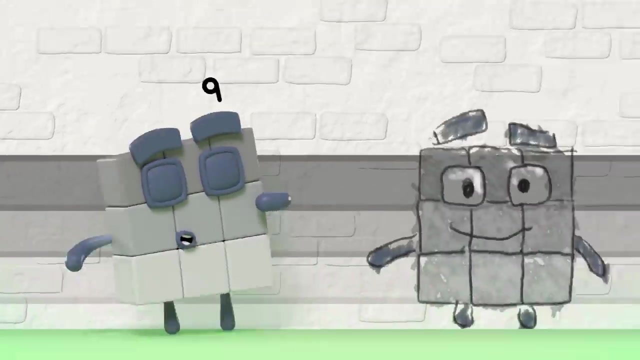 you can fill in the space. that's the difference one. and if the difference won't pop into your head, you can count another. blocks in place: one, two, three, four, five, five. the difference is five. so what's the difference? nine nine minus six equals three. that's the difference three. 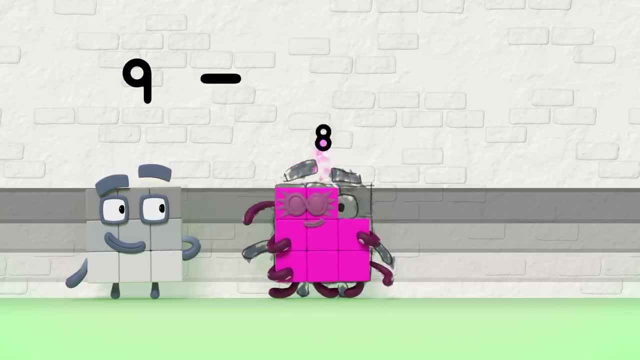 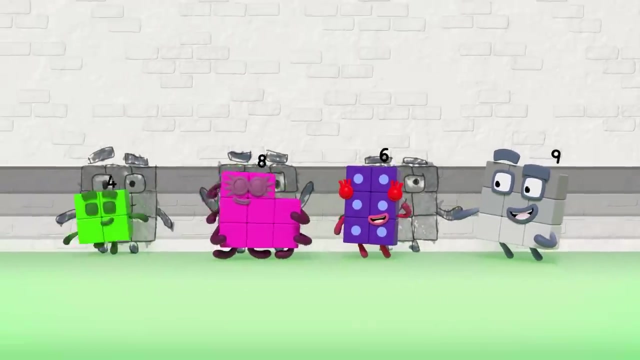 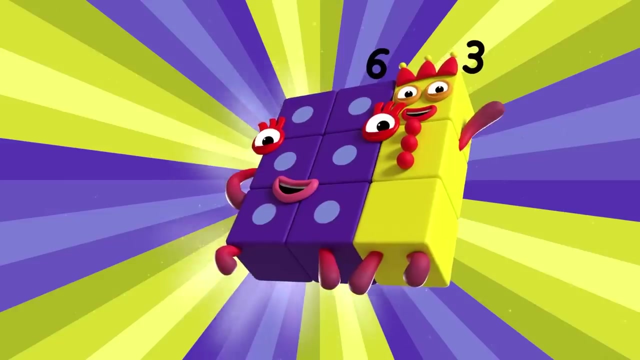 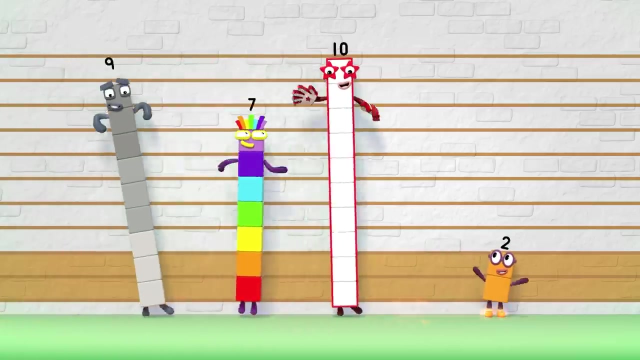 nine minus me equals one. that's the difference. one. nine minus four equals five. that's the difference. five. so make up the difference and everyone will see what the difference is between you and me. seven: I'd love to be you, but I'm much too big. 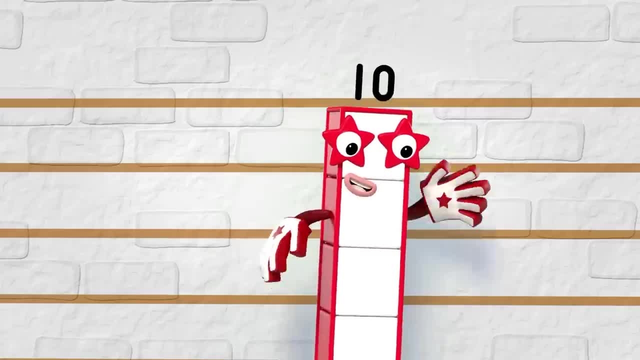 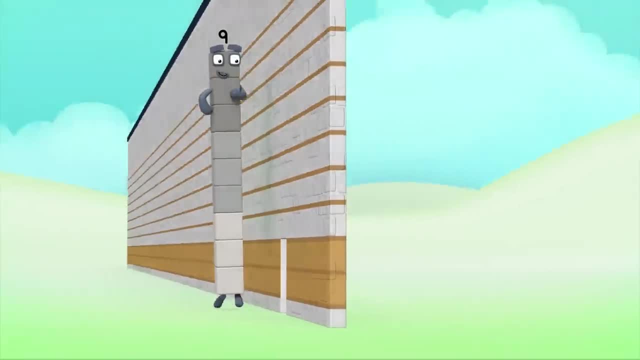 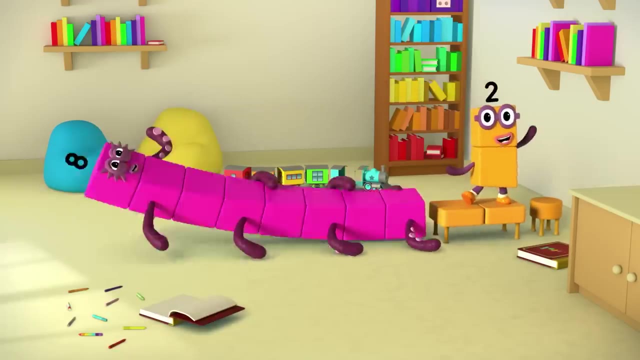 We need to lose something, but what? I'd love to have some of your talent. What makes you two and someone? we're not. I could walk through a door, That's the difference. I could get into bed, That's the difference. And if the numbers won't pop into your head? 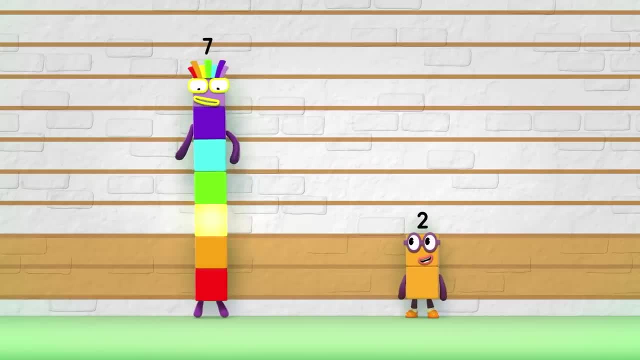 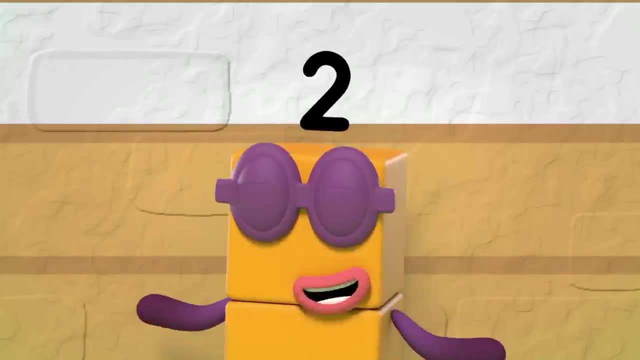 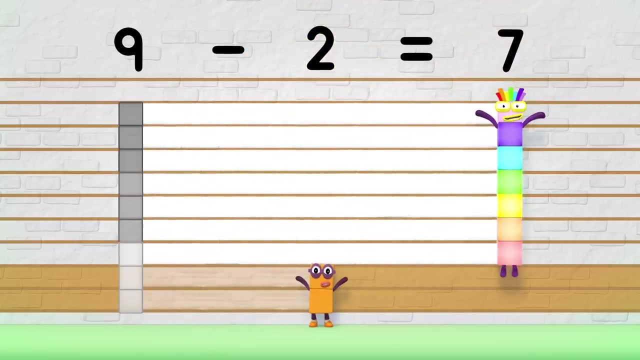 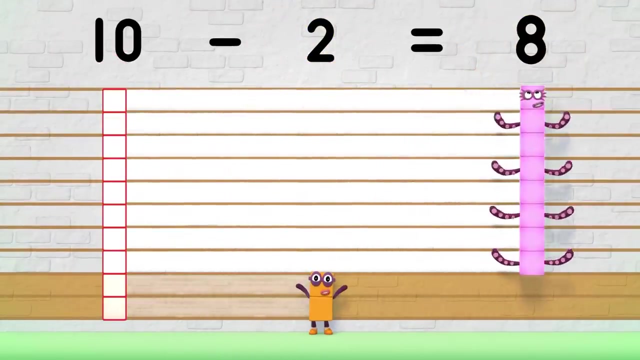 You can count the extra blocks instead: One, two, three, four, five, Five. The difference is five. So what's the difference? Nine minus two equals seven. That's the difference. Seven Ten minus two equals eight. That's the difference. Eight Seven Minus two equals five. 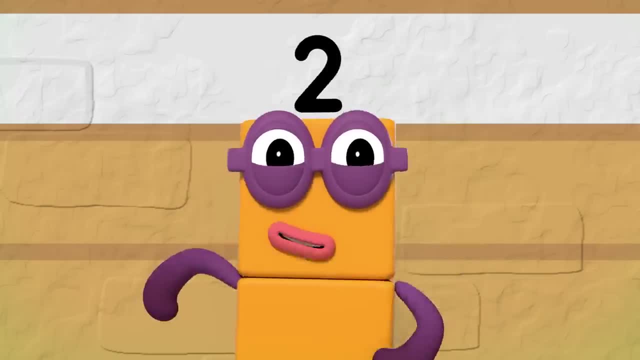 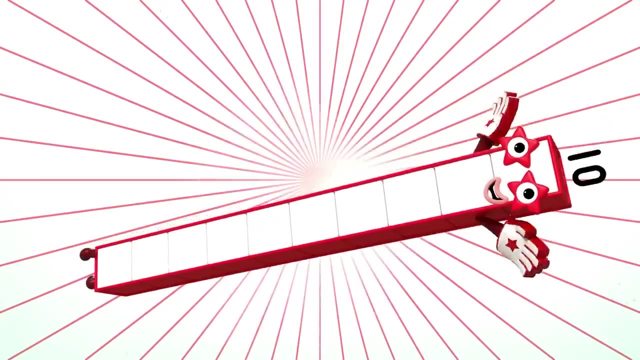 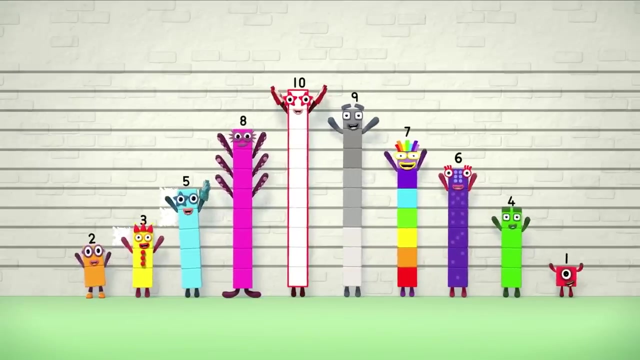 That's the difference Five. So take off the difference And everyone will see what the difference is Between you and me. We all have our place when we're different. You have to admit we've come far. We're all friends here, but we're different And the differences between us. 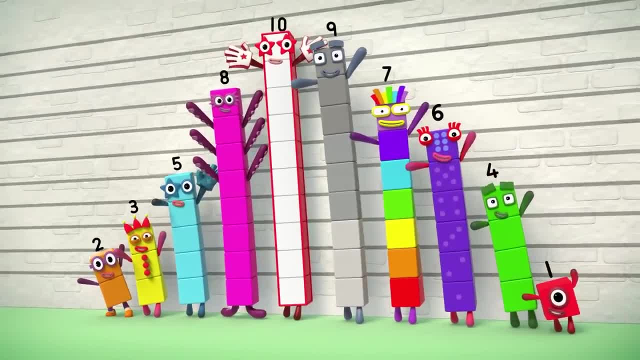 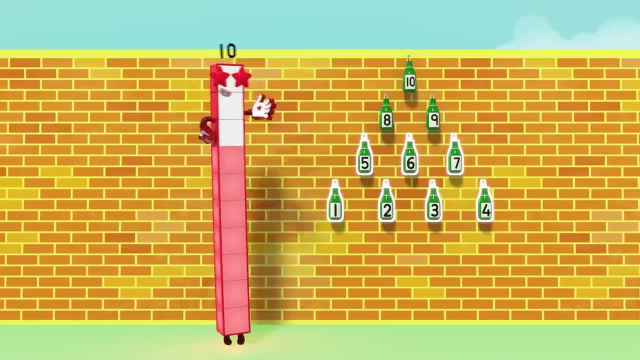 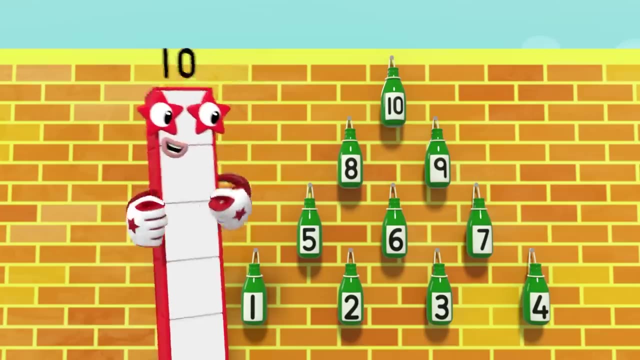 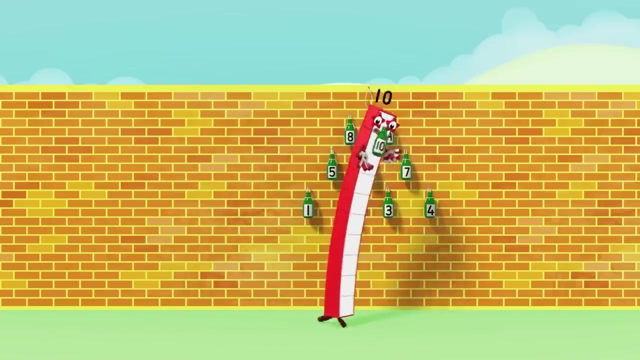 Make a difference. That's who we are: One, two, three, four, five, six, seven, eight, nine, ten, Ten green bottles. Ten green bottles hanging on the wall, Ten green bottles hanging on the wall. But if one green bottle should accidentally fail, 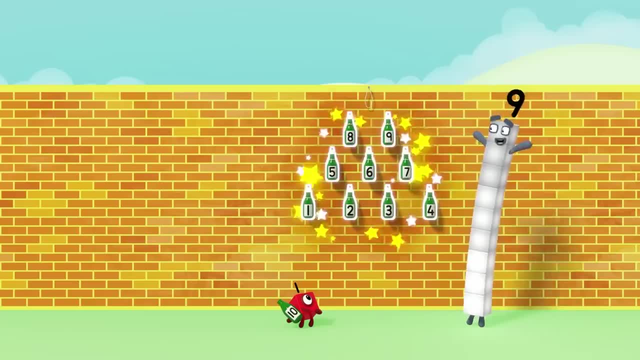 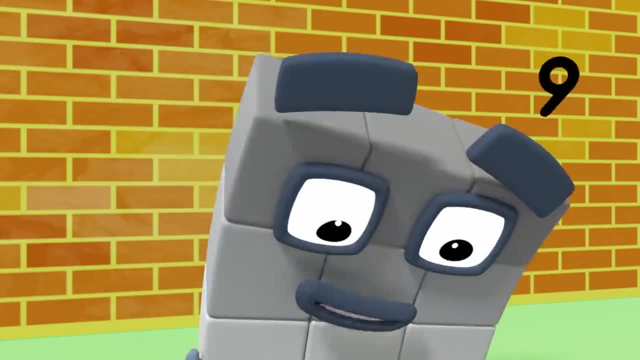 There'll be one, two, three, four, five, six, seven, eight, nine, ten green bottles. Ten green bottles hanging on the wall. Better move these nine before they fall. They're not safe up there. Nine green bottles, safely on the floor. 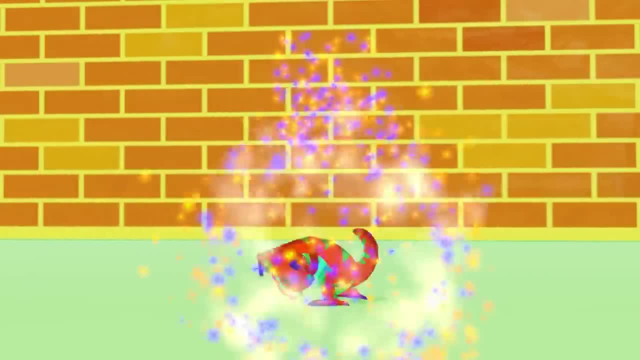 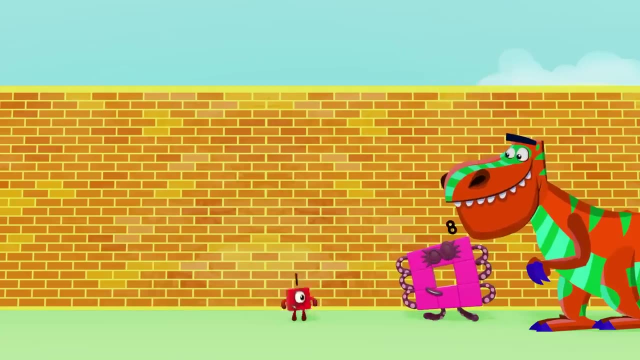 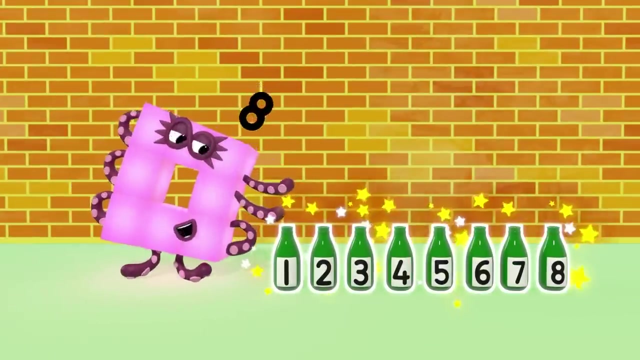 Nine green bottles safely on the floor. Oh, oh, uh, uh, uh, ah, achoo. But if one green bottle becomes a dinosaur, There'll be one, two, three, four, five, six, seven, eight, Eight green bottles not safe on the floor. 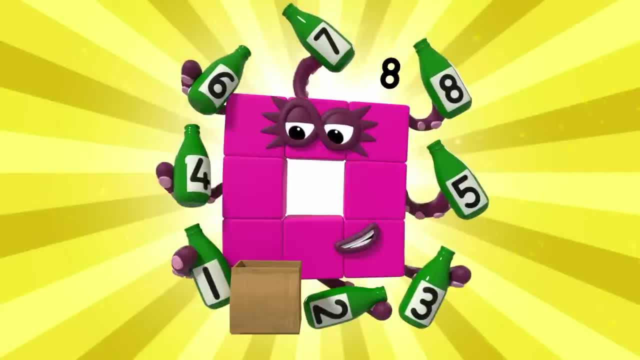 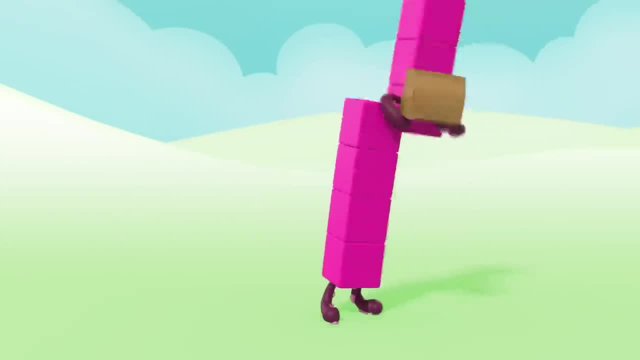 Octoblock high. One, two, three, four, five, six, seven, eight high. Eight green bottles hiding in a box. Eight green bottles hiding in a box. But if one green bottle is stolen by a fox, Hey, There'll be one, two, three, four, five, six, seven. 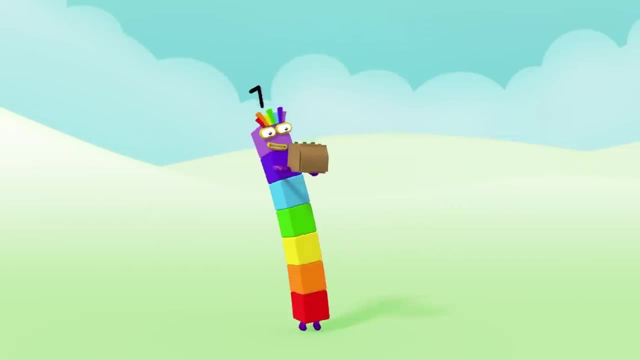 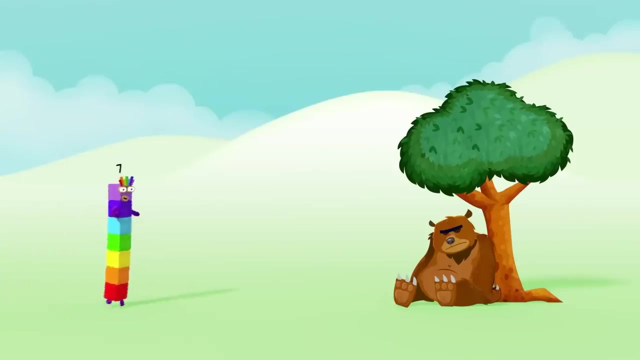 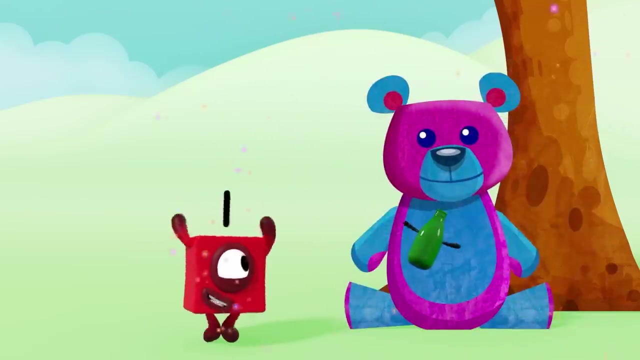 Seven green bottles hiding in a box. That was lucky, Ooh. Seven green bottles hiding in a box. Eight green bottles flying through the air. Seven green bottles flying through the air. But if one green bottle should wake a grizzly bear, What I mean? hug a teddy bear. 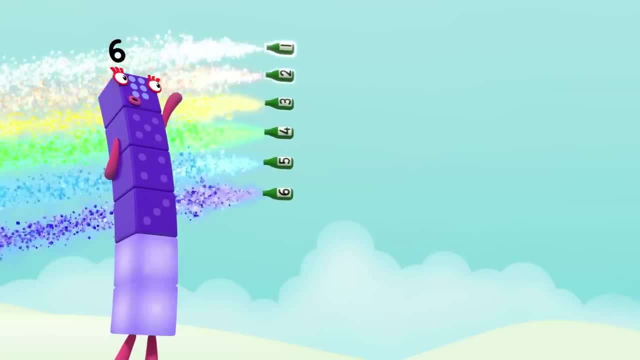 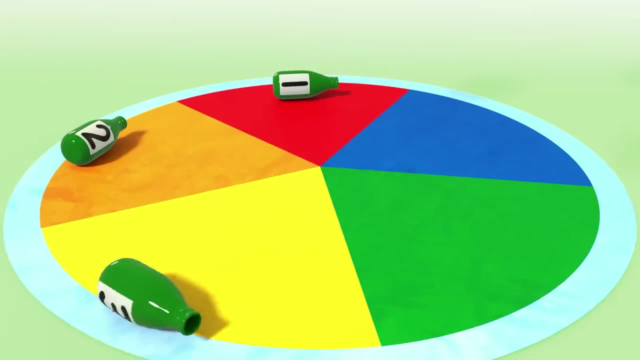 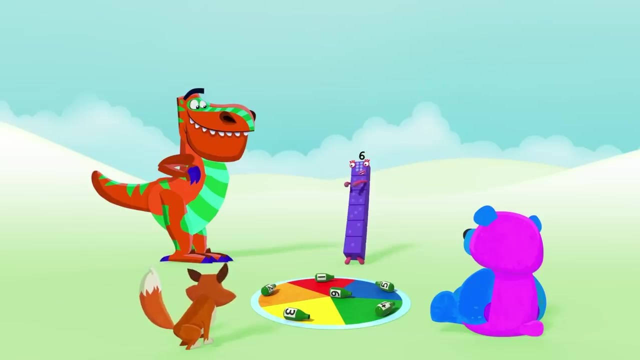 Phew, There'll be one, two, three, four, five, six, Six green bottles falling through the air. Six is my name. let's play a game, And this game goes like this: Six green bottles flying through the air. Six green bottles flying through the air. 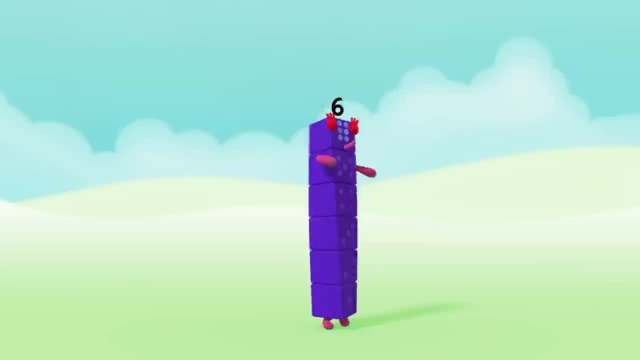 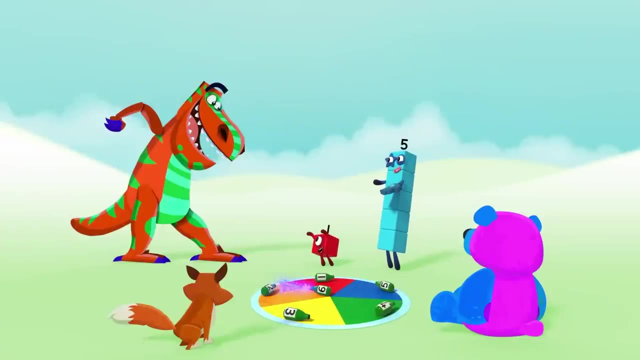 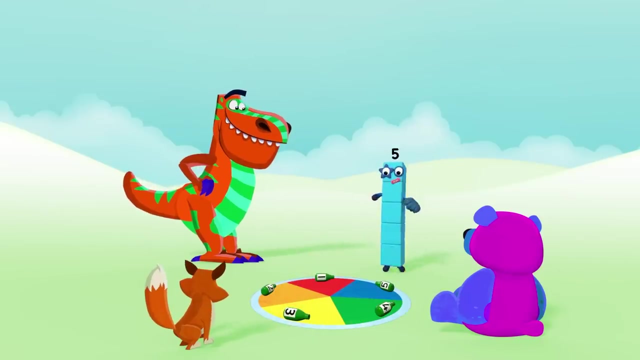 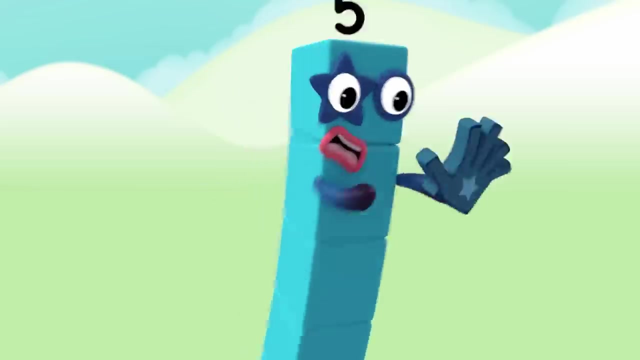 Six green bottles lying on the ground. Six green bottles lying on the ground, And if one green bottle spins around, Whoa, You win. There'll be one, two, three, four, five, Five green bottles lying on the ground. Yeah, Five green bottles rolling down the hill. 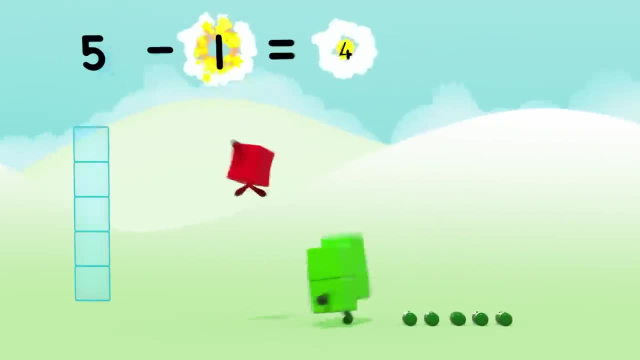 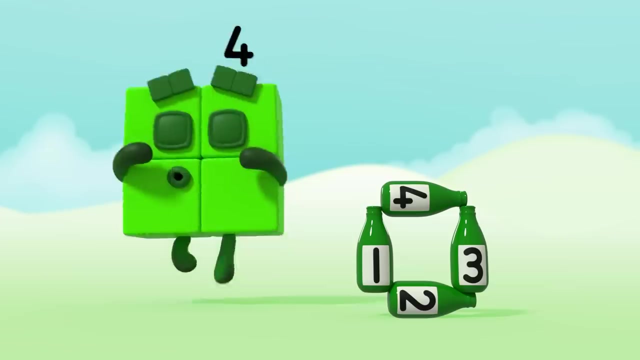 Five green bottles rolling down the hill, But if one green bottle should grow a daffodil, There'll be one, two, three, four, five green bottles Rolling down the hill. Four green bottles standing in a square. Four green bottles standing in a square. 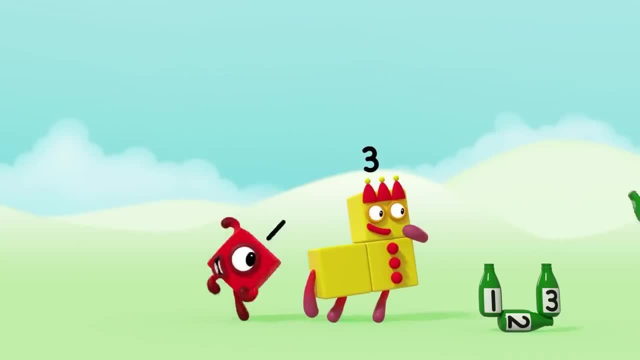 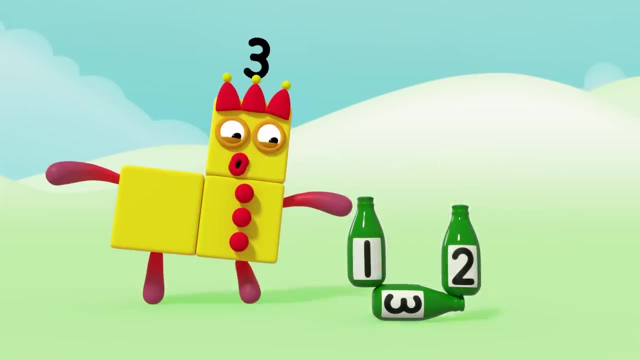 But if one green bottle should run to the bear, There'll be one, two, three, four, five green bottles. There'll be one, two, three, four, five green bottles. Three green bottles standing in a triangle: One, two, three. 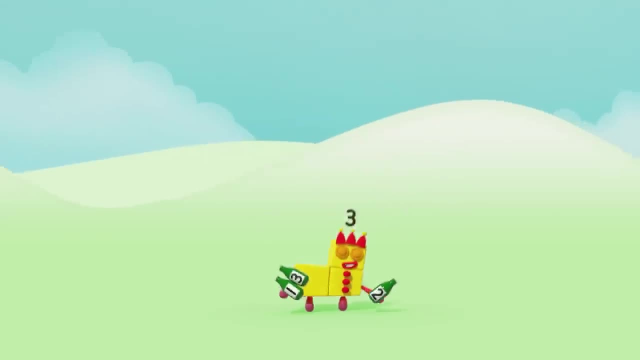 Three green bottles spinning in the sky. Three green bottles spinning in the sky, But if one green bottle should pop its wings and fly, There'll be one, two, three green bottles spinning in the sky. Come back. Two green bottles floating out to sea. Two green bottles floating out to sea. 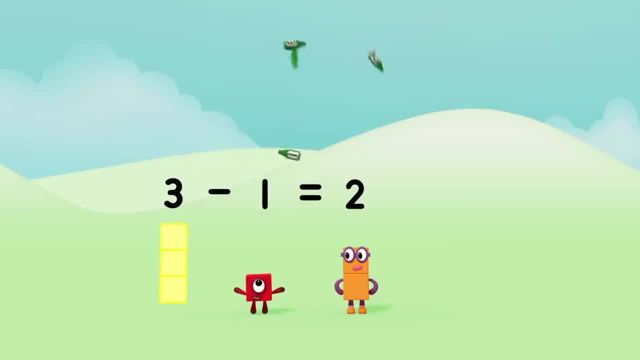 But if one green bottle should pop its wings and fly, There'll be one, two, three green bottles spinning in the sky. Come back, Two green bottles floating out to sea, Two green bottles floating out to sea. Two green bottles floating out to sea. But if one green bottle should pop its wings and fly, 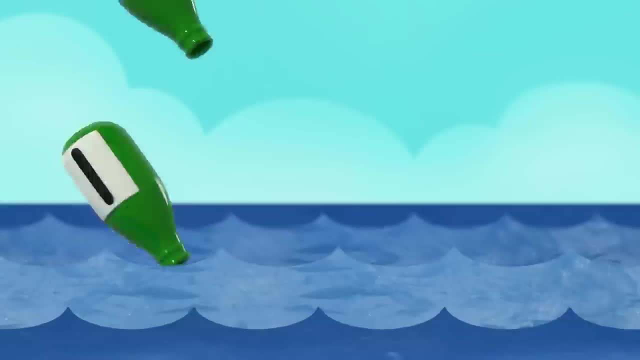